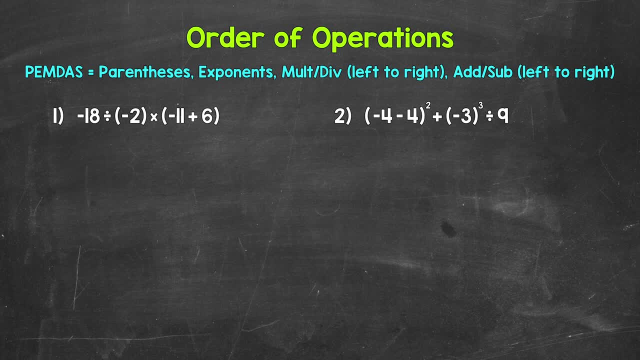 Do we have anything to do with in parentheses? Yes, we have negative 18 divided by negative 2 times, and then in parentheses, negative 11 plus 6 end parentheses. So let's start there. Negative 11 plus 6 gives us negative 5.. So we start at negative 11 and add 6.. 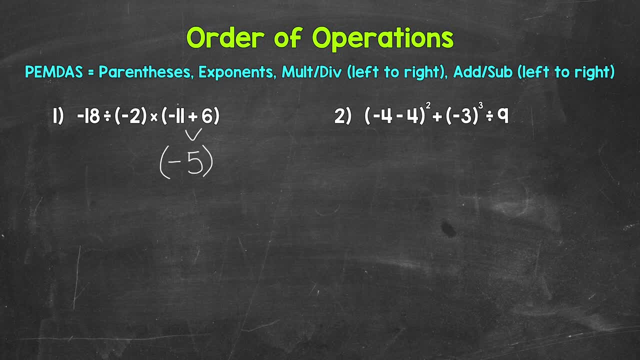 So we are increasing in value by 6 and get negative 5.. So now we can bring down everything we did not use and go from there. Now we have negative 18 divided by negative 2 times, and then in parentheses negative 11 plus 6, end parentheses. So we have negative 18 divided by negative 2 times. 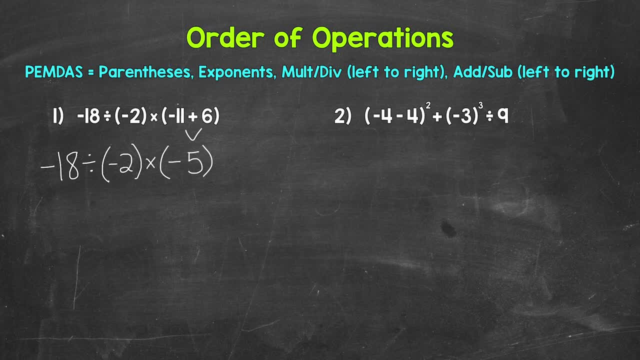 negative 5. And you'll notice I'm keeping some of the negatives within parentheses. That helps us stay a little more organized and we don't confuse any negatives for subtraction or forget any of the negative signs. It makes the negatives a little more clear and again helps us stay organized. 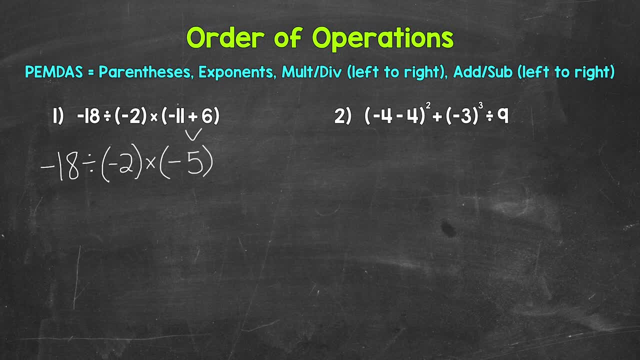 I left the negative 5 and the negative 6 in parentheses. So we have negative 8 and the negative 18 without parentheses, because it's in the front and the negative is clear. But we can definitely put it in parentheses as well if we would like. So let's continue to work through the order of 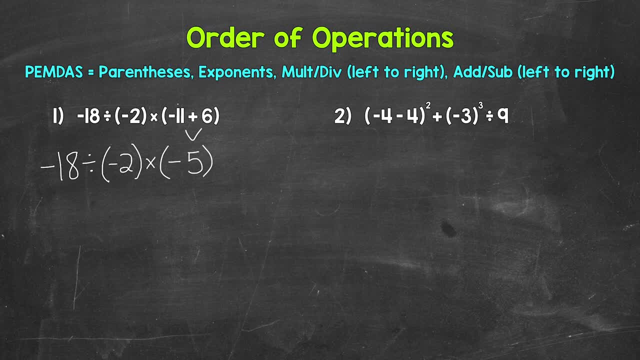 operations Anything to do with in parentheses. No, Any exponents, No, Any multiplication or division. Yes, We actually have both multiplication and division. Multiplication and division are the same priority, So we work from left to right. When working from left to right, we have division first. 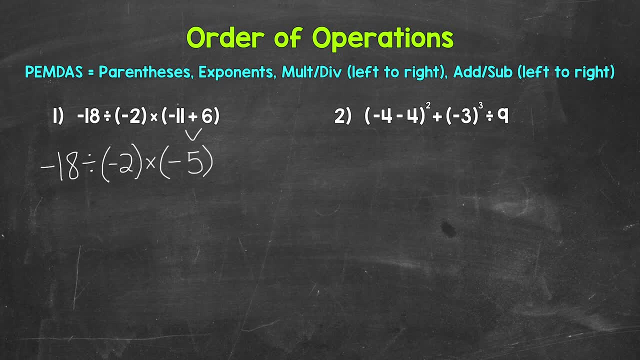 We have negative 18 divided by negative 2. So we have a negative divided by a negative. That gives us a positive. So negative 18 divided by negative 2 is 9.. A positive: 9. Then we can bring down everything we did not use. So times negative 5.. 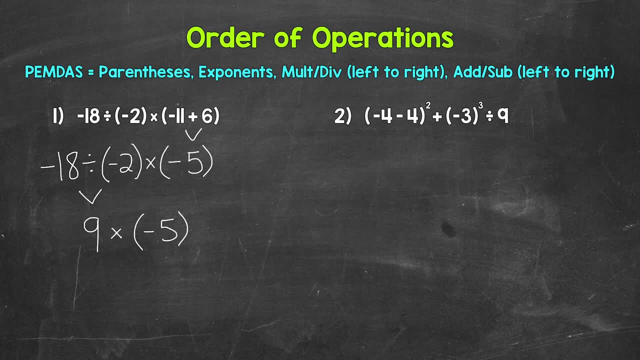 And now we have 9 times negative 5.. A positive times a negative equals a negative. So 9 times negative 5 is negative 45. And this is our final answer: Negative 45.. Let's move on to number 2. 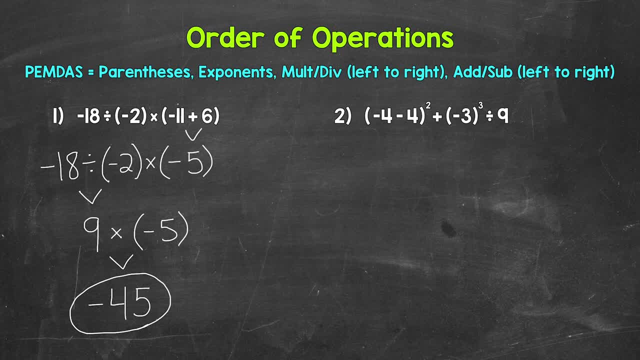 where we have in parentheses negative 4 minus 4 end parentheses, And we are squaring what we get within those parentheses, Plus negative 3 cubed divided by 9.. So let's work through the order of operations. Do we have anything to work through within parentheses? Yes, We have negative. 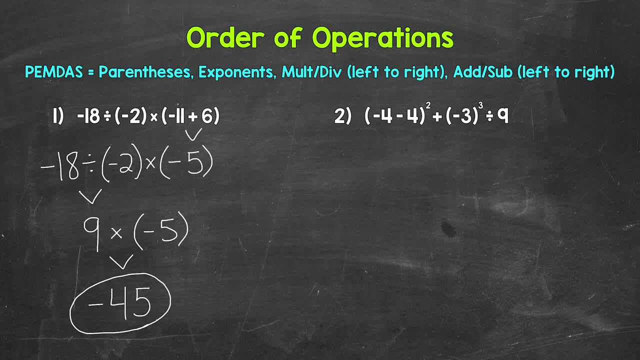 4 minus 4.. So let's start there Now. remember one thing we can do: when we have subtraction, we can add the opposite, And that can help when we have problems involving negatives. So let's add the opposite. Here we have negative 4 plus, and then the opposite of positive 4 is negative 4.. So negative 4 plus. 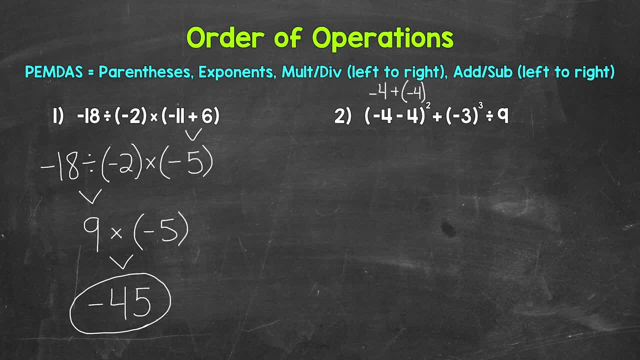 negative 4, or negative 4 minus 4.. That gives us negative 8.. And we need to keep that negative 8 within parentheses because we are squaring this result, We are squaring what we got within the parentheses. It's very important to keep that negative result- negative 8- in parentheses because, again, we are 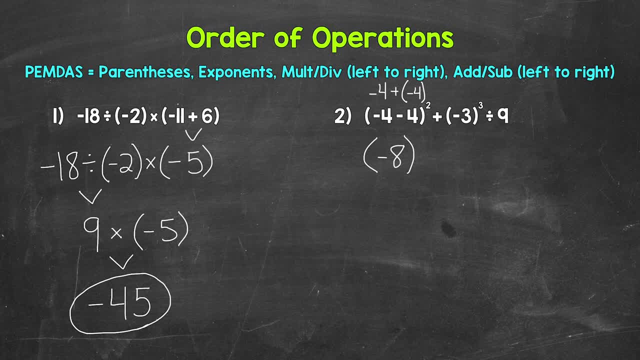 squaring it. We have an exponent. Now, remember- and I'm going to come to the side here- Negative 8 squared is different than if we do not have the parentheses. Negative 8 squared with parentheses means negative 8 times negative 8.. 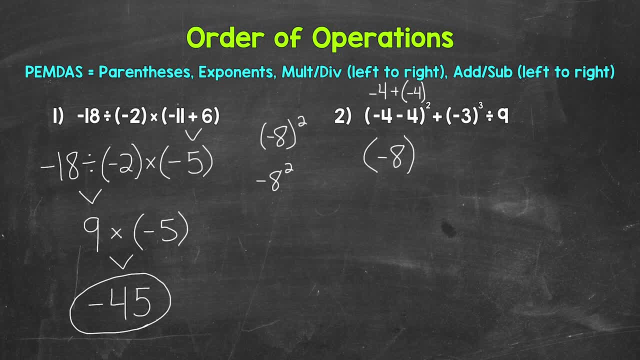 Which equals 64. The negative is included with the exponent. Without the parentheses, that means 8 times 8, which is 64. The exponent is only applied to the 8. And then we have the negative sign in front. So without the parentheses, that equals negative 64. Now, if you need more of an explanation as far as 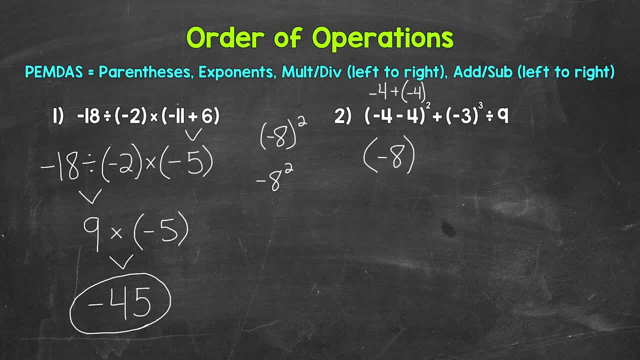 the negative sign in front, Then you can use the negative sign in front And then you can use the difference between those. I go into more detail in another video. That link is in the description. So we have negative 8 squared plus negative 3 cubed divided by 9. So now we have negative 8. 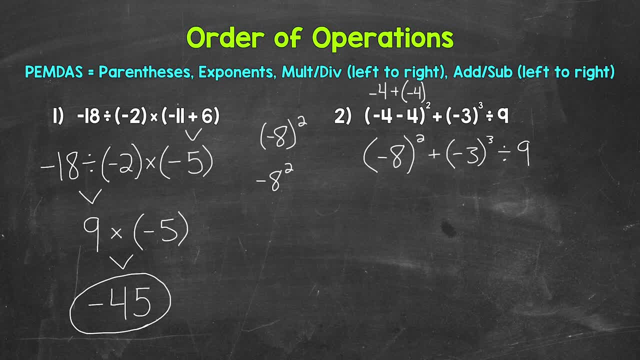 squared plus negative, 3 cubed divided by 9.. Do we have anything to work through? within parentheses? No. Do we have any exponents? Yes, we have two exponents. So let's start with negative 8 squared, Which means negative 8 times negative 8.. So a negative times a negative, A negative times a negative equals a. 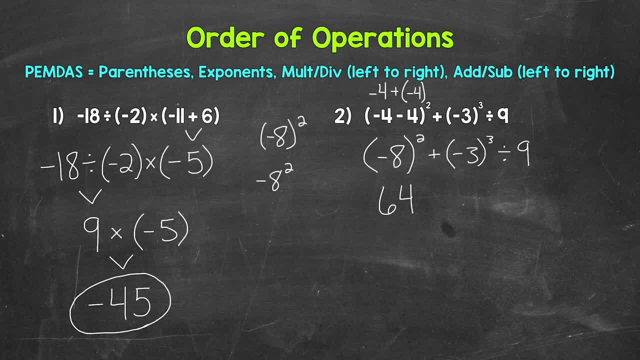 positive. So this gives us positive 64. And we will go one step at a time here. So let's bring down everything we did not use And now we have 64.. So we have 64 plus negative 3 cubed divided by 9.. So now we can do negative 3 cubed. That means 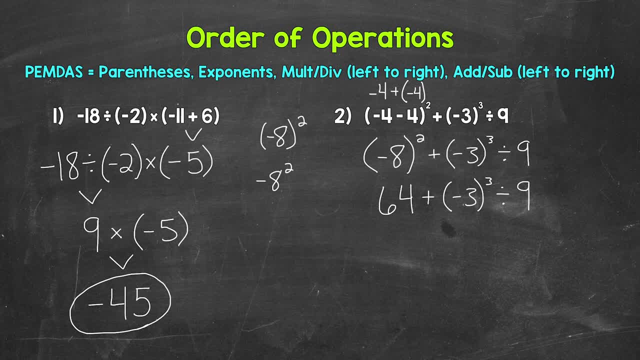 negative 3 times negative, 3 times negative 3. Negative 3 times negative. 3 is positive 9. So we have positive 9 times negative 3. That gives us negative 27.. So we have negative 27.. Bring down. 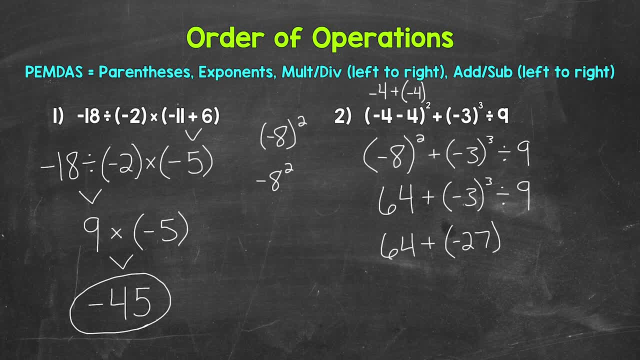 everything We did not use. And now we have 64 plus negative 27 divided by 9.. Now, just as a quick recap, as far as negative 3 cubed and how we got negative 27.. I'm going to come to the side here. So we had 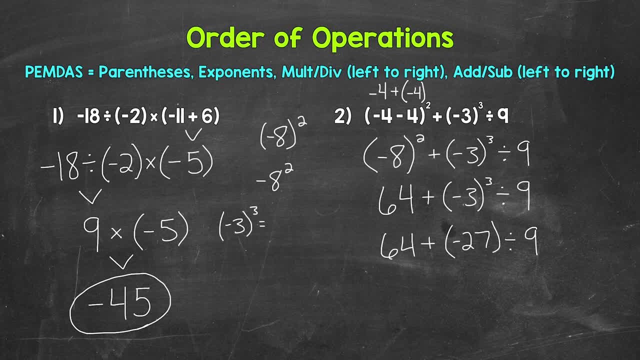 negative 3 cubed, Which means negative 3 times negative, 3 times negative 3 cubed. So we have 64 plus negative 27 divided by 9.. So we have 64 plus negative 27 divided by 9.. So we have 64 plus negative 27. 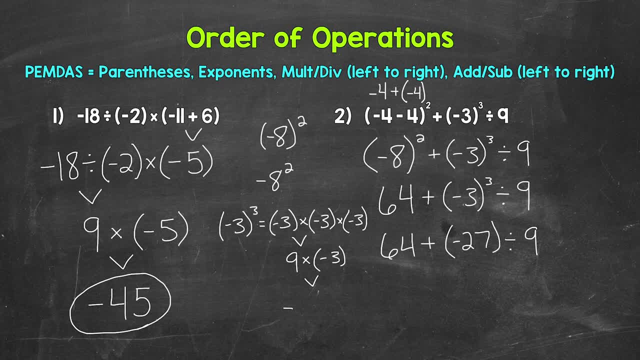 A positive times a negative equals a negative. So nine times negative three equals negative 27.. So now, as far as the order of operations, we have 64 plus negative 27 divided by nine. Do we have anything within parentheses that we need to work through?